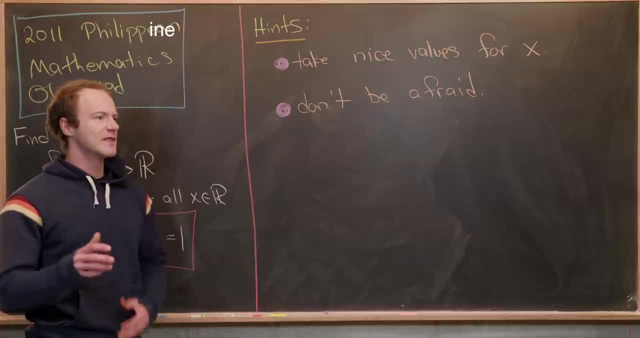 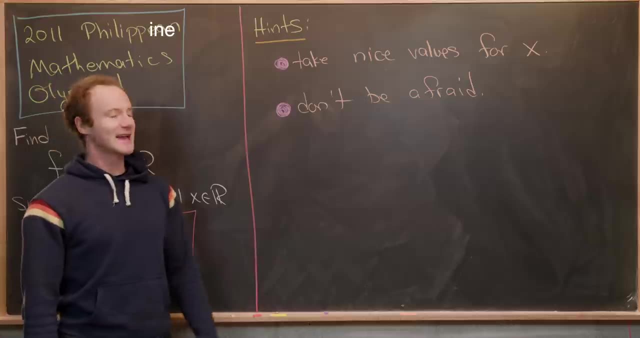 Those are nice values for x, and really the nice values depend on the structure of the functional equation. So keep that in mind as well. And then my second hint. well, this is really a good hint for all math problems, and that is: don't be afraid, Don't be afraid of working on it for a long time. 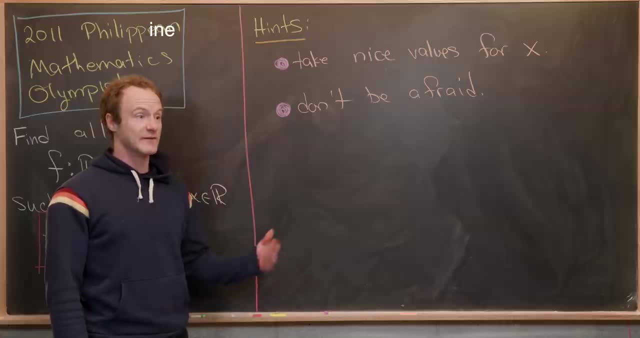 and possibly failing, and also don't be afraid of coming up with a solution that seems wrong but might be correct. Okay, so let's go ahead and look at a solution. So hopefully those hints were helpful. Now we're ready to jump into a solution and we'll jump into. 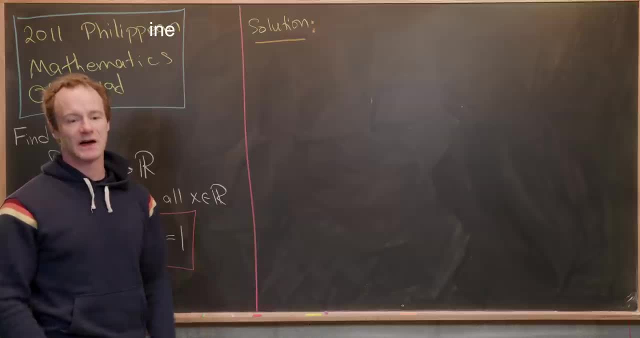 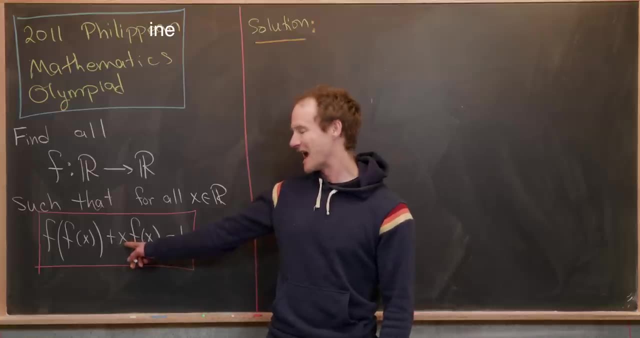 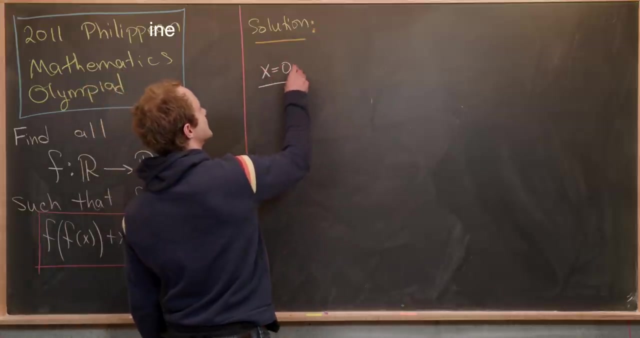 our solution using our first hint, which is to take nice values for x, And I think x equals 0 is maybe the nicest value to start off with, because we have this x which is floating outside of the function. Okay, so let's see what we get if we set x equal to 0. So x equal to 0 into the functional equation. 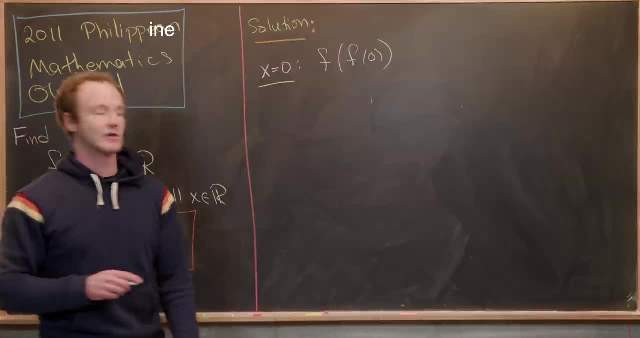 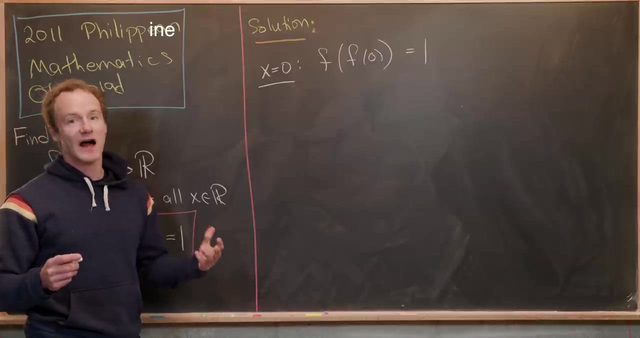 gives us f evaluated at f of 0.. Plus 0 times f of 0 equals 1.. But we can clearly get rid of that 0 times f of 0. So we immediately have a value for the function. Now it's not really that helpful. the value at the 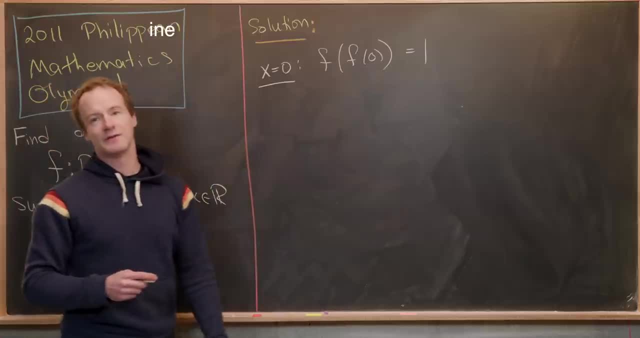 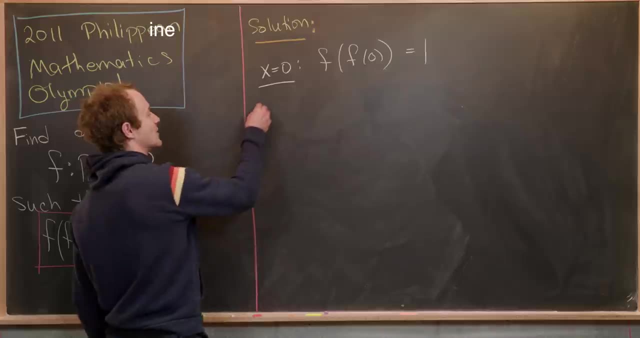 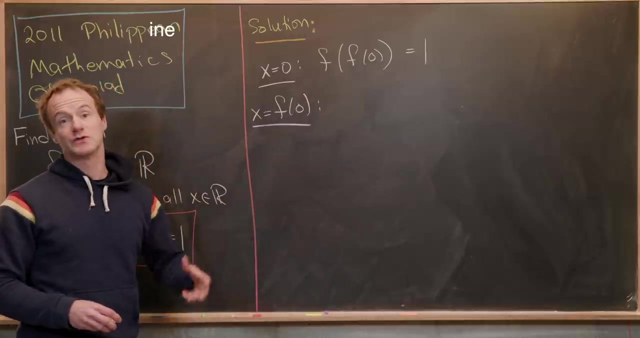 moment, because we know f evaluated at f of 0 equals 1.. But at least it's a start, And this gives us actually a great hint that our next substitution should be x equals f of 0.. Since we know how to decompose repeated applications of f on the number 0. 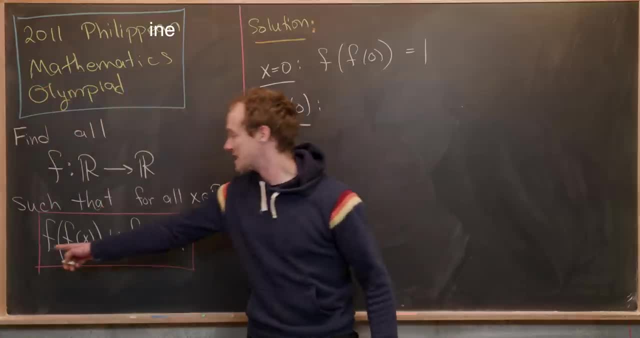 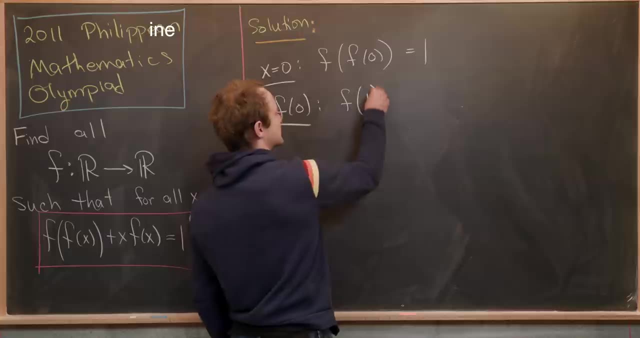 Okay, so let's see what that gives us. So that's going to give us f of f, of f of 0. But we know that's going to be f of 1.. So here let's write that down and then we will remind. 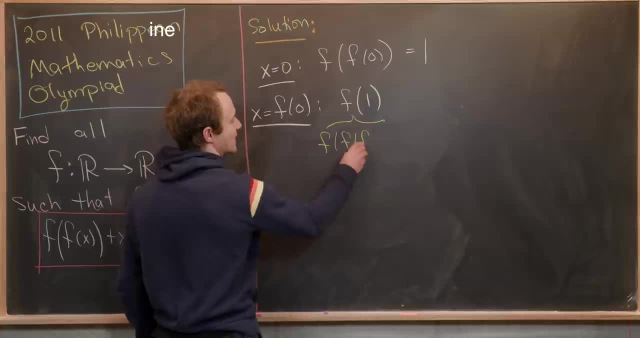 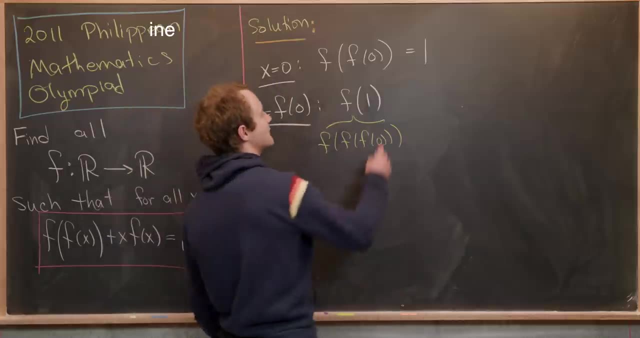 ourselves that that comes from taking f of f of f of 0 like that Great. and that's the first term right here. The next we'll have that this is f of f of 0 plus x. in this case, x is f of 0 times f of x, But f of x is going to be f of f of 0. 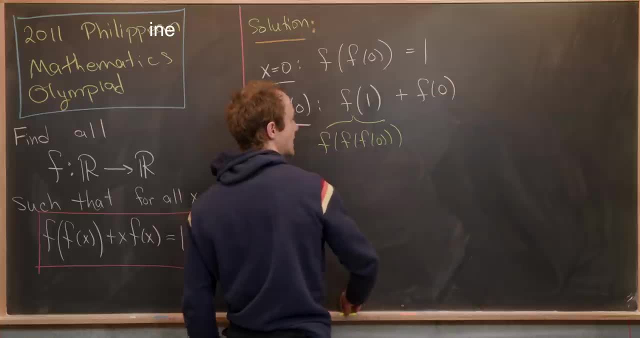 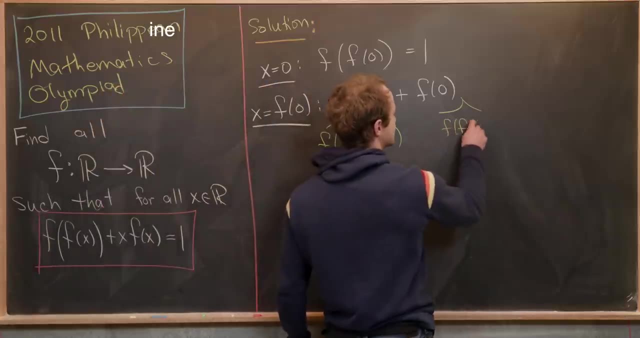 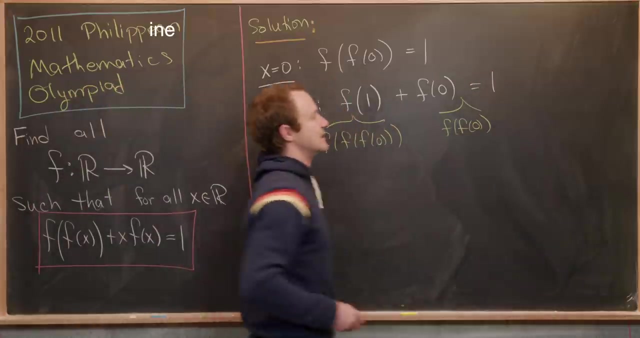 But that's just 1.. So we can just write that as times 1.. And keep in mind that this 1, which is hidden right here, is actually f of f of 0. And we know that value from our first step. Okay, so next, we know that this is equal to the number 1.. 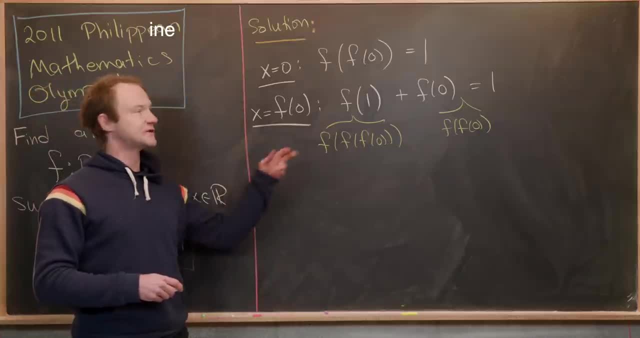 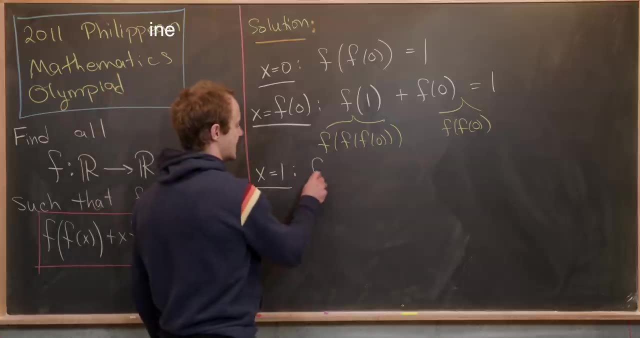 We will set x equal to 1.. And the motivation for that is: we see f of 1 right here. So let's see what we get from setting x equal to 1.. So that's going to give us f evaluated at f of 1 plus f of 1 times. 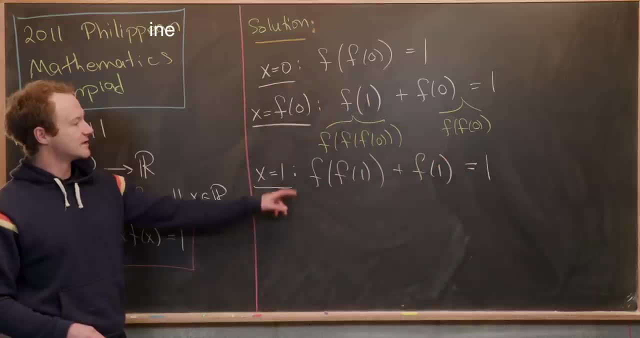 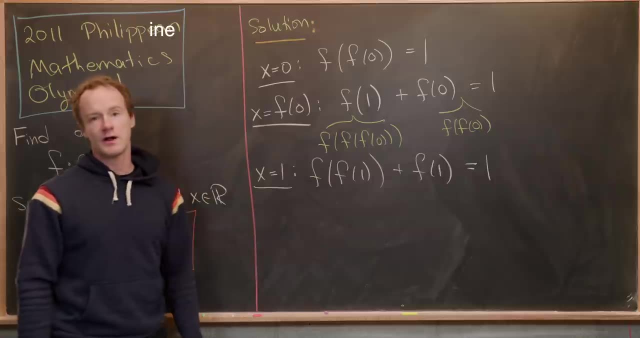 1 from this right here equals 1, like that. But notice, this gives us a nice system of equations where we can think about our three variables as being f of f of 1, f of 1 and f of 0.. But now by: 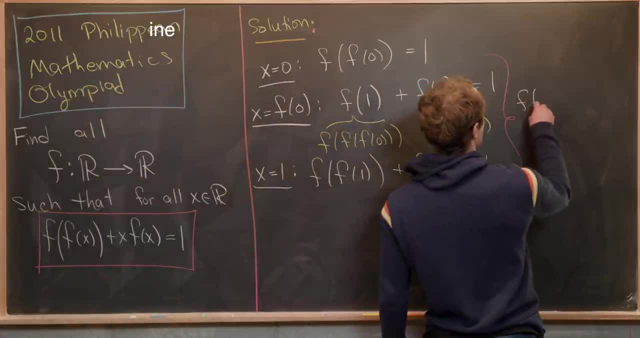 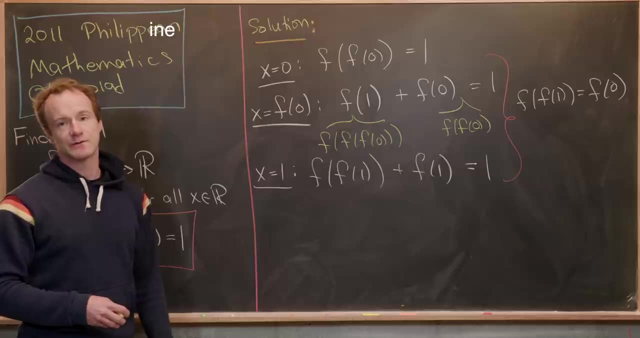 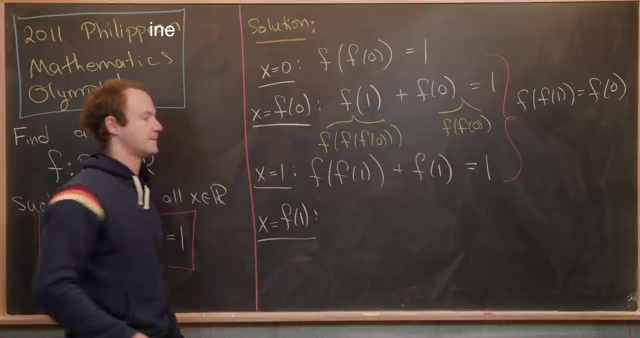 subtracting these two equations, it's pretty easy to see that f evaluated at f of 1 is equal to f evaluated at 0. And that also gives us some motivation for what our next substitution should be. Perhaps it should be: x equals f evaluated at 1.. So let's see what we get throwing that into. 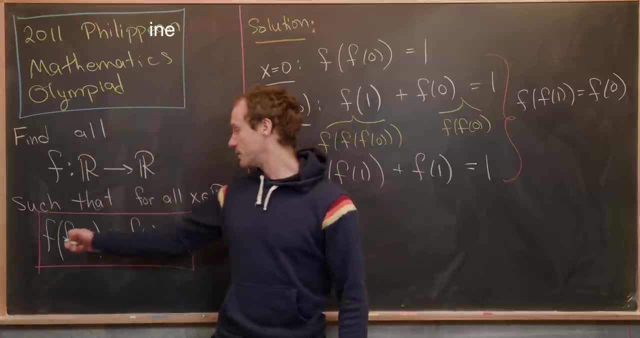 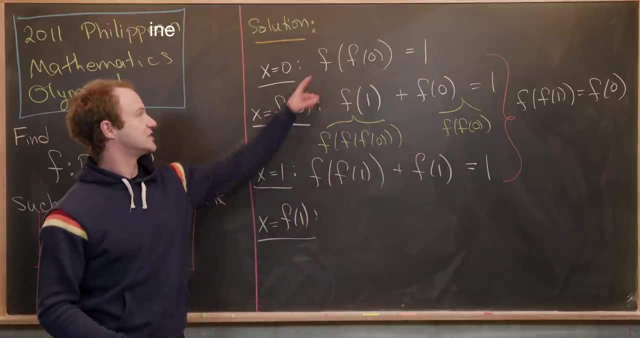 our functional equation. So our first object will be f of f of f of 1.. But notice, f of f of 1 is 0.. In fact it's just f of f of 0, which is 1.. So let's write that down and then we'll expand this. 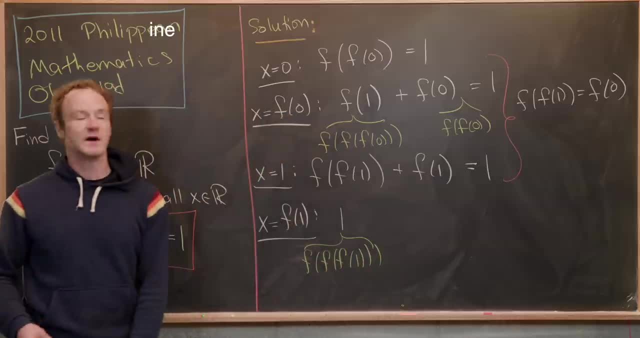 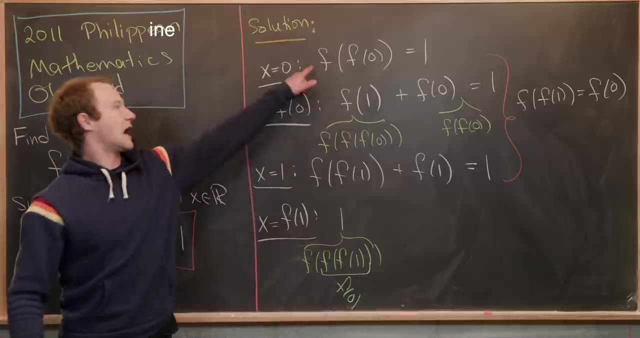 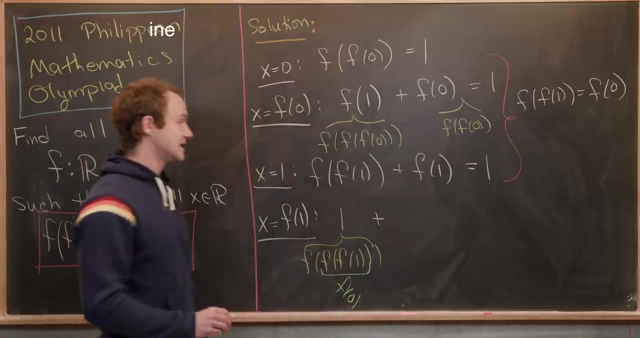 as it looks exactly in the functional equation, where again we use the fact that this inner part is f of 0. And then our original equation tells us that is equal to 1.. Okay, good, But now this is going to be plus f of 1, that's x times f of f of 1.. 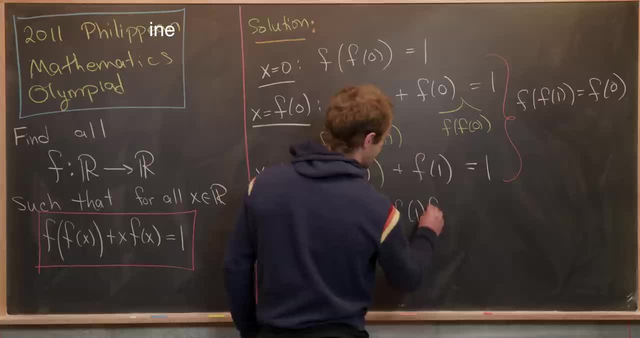 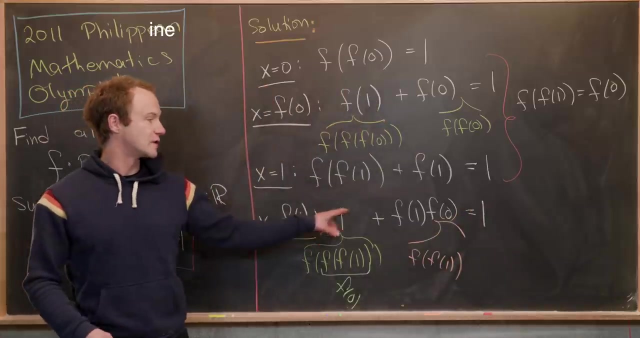 But that is f of 0 from this here. so we have f of 1 times f of 0. Again, this term right here comes from f of f of 1.. And then over on the right hand side of the equation we have this is equal to 1.. But now notice, the 1's will cancel from both. 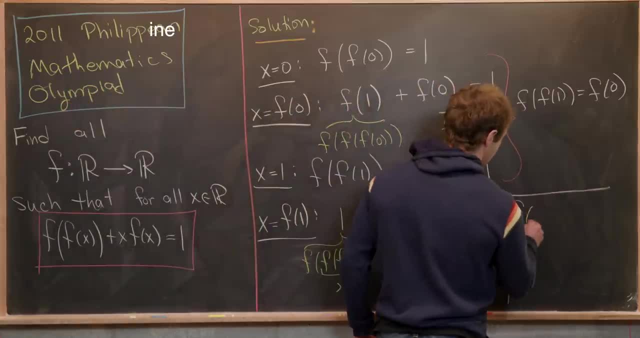 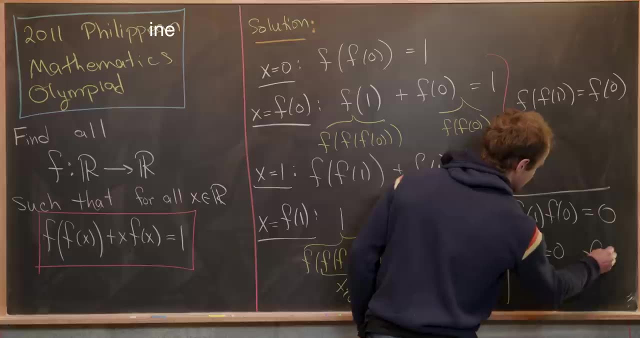 sides of the equation And we end up with f of one times f of 0 equals 0. Which brings us to 2 cases: F of 1 equals 0- Incredibly. let's see what we can do here. We have 2 cases: fe of 1 x, f of 0 equals 0. 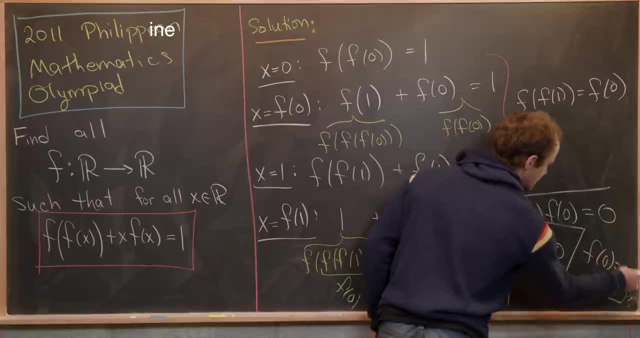 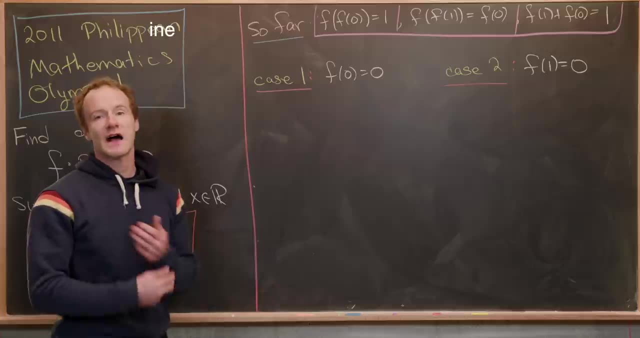 zero, or f of zero equals zero. So I'll actually clean this board up and we'll start with the necessary facts to finish it off, including those two. So in the last board we derived the following equations involving evaluating this function at zero one, and then multiple compositions of this: 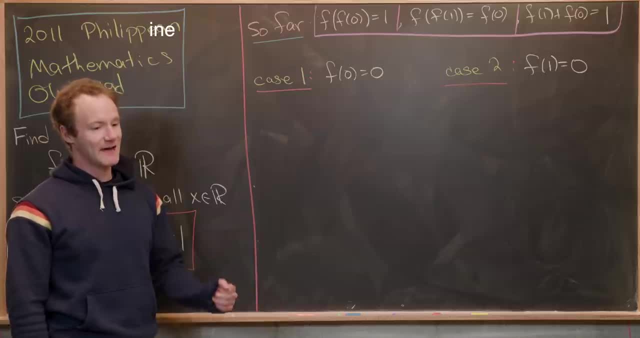 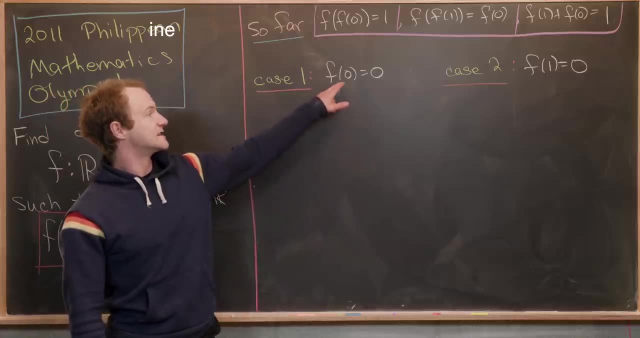 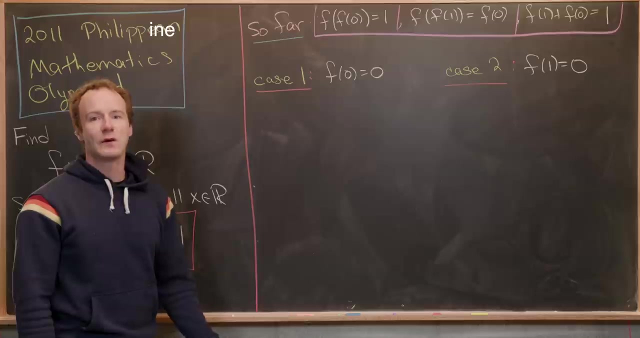 function at zero and one. We also figured out that f of zero times f of one was zero, so that means one of them was at least zero. So here we'll break this into two cases. The first one is f of zero is zero, and the second case is f of one equals zero, And we'll see what each of these cases imply. 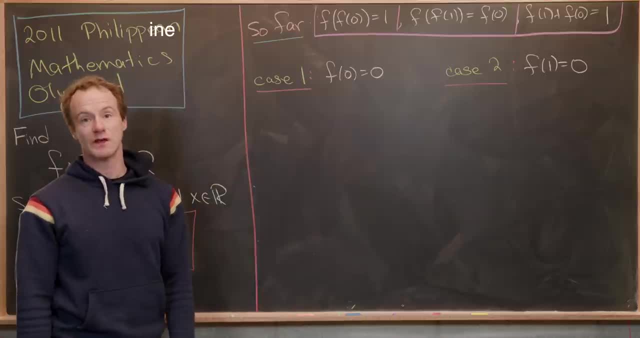 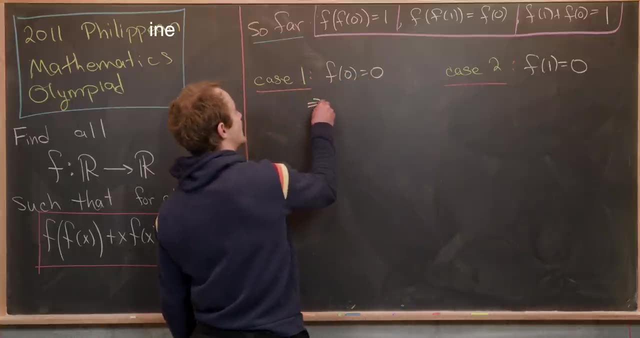 So we'll start off with this part right here, which is f of zero equals zero. So notice, if f of zero equals zero, by this equation right here we have f of one equals one. Okay, but then we'll break this into two cases. The first one is f of zero equals zero, and the second case is: 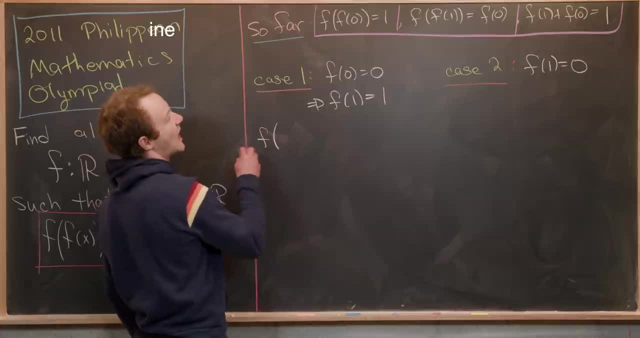 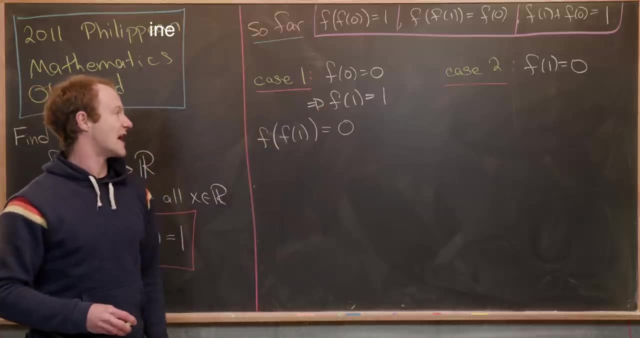 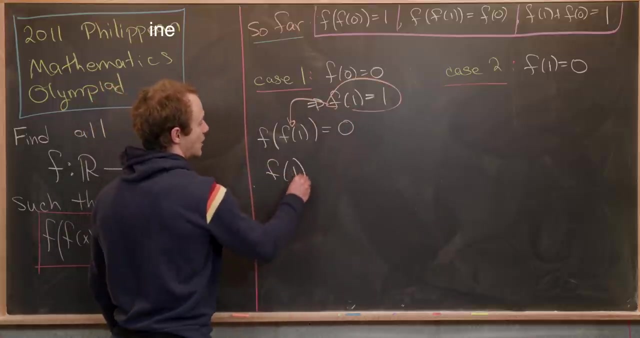 by this equation right here we have f of f of 1 equals f of 0, which is 0. Okay, but also we have f of 1 equals 1, so we can plug this in here and we see that f of 1 equals 0. So simultaneously, 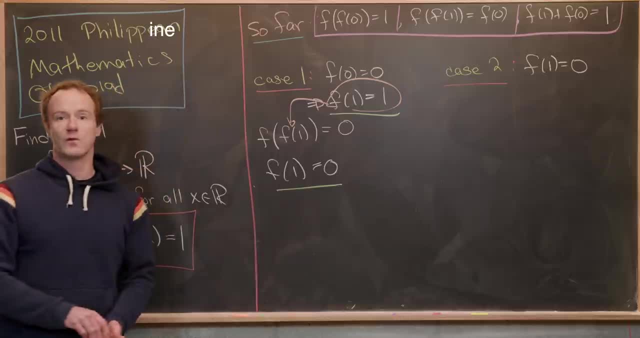 we have f of 1 equals 1 and f of 1 equals 0. So that's a contradiction which means this case is impossible. So let's jump to the second case, and that's the case when f of 1 equals 0.. 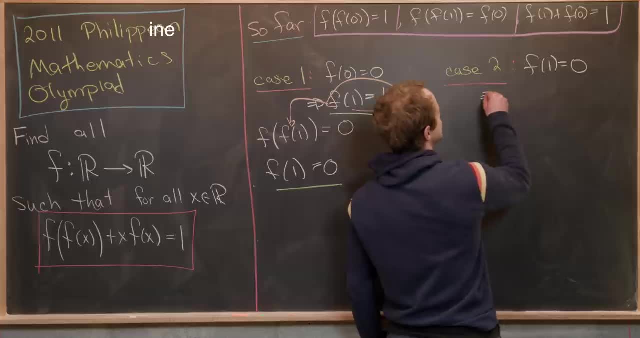 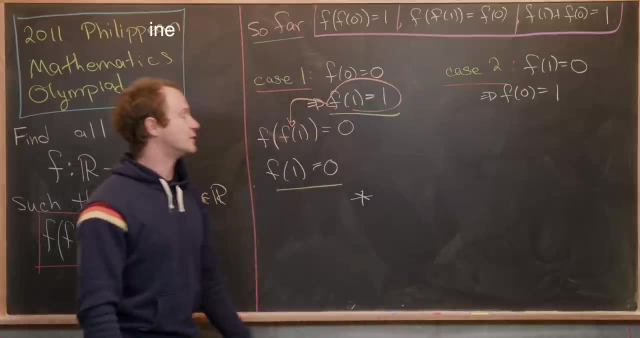 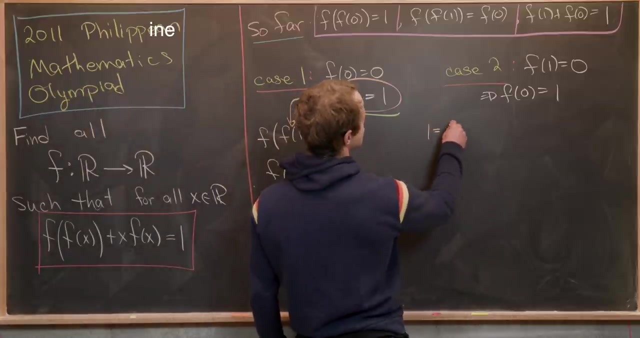 So again, if f of 1 equals 0, that tells us that f of 0 equals 1. by this equation right here. But now combining these two equations with this one right here, we'll see that something goes wrong. So notice that we'll have: 1 equals f of f of 0 equals f of 1. 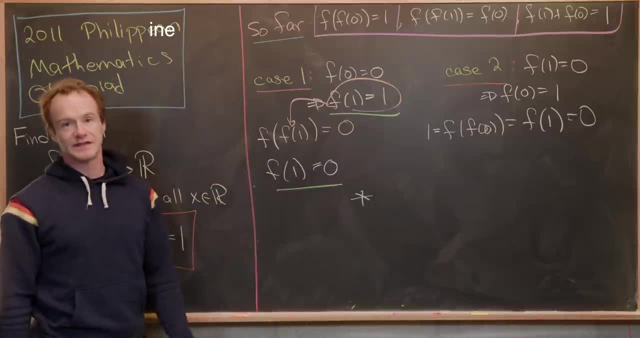 equals f of 1 equals 0. So that's a contradiction which means this case is impossible. So let's jump to the second case: equals zero. so again we get one equals zero, a similar contradiction to what we got right here. so in other words, we've got a contradiction. so the two only possible cases brought us to a. 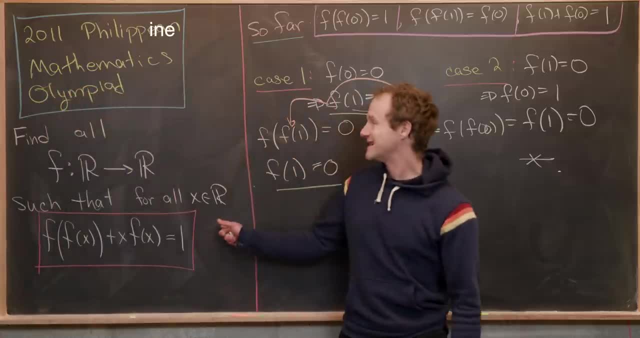 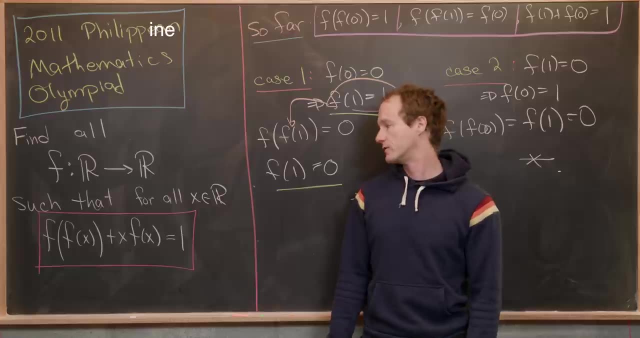 contradiction, which means finding all functions. satisfying this rule is impossible. well, we did find all of the functions. it's just that there are no functions, and that's a good place to stop.